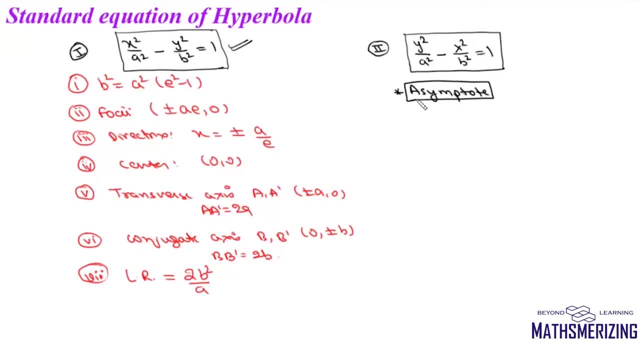 In case of a hyperbola, we do have two special lines which we call asymptotes of a hyperbola. Now, basically, what is an asymptote? So asymptote is essentially a line which meets the curve at infinity. So suppose we have this hyperbola which is 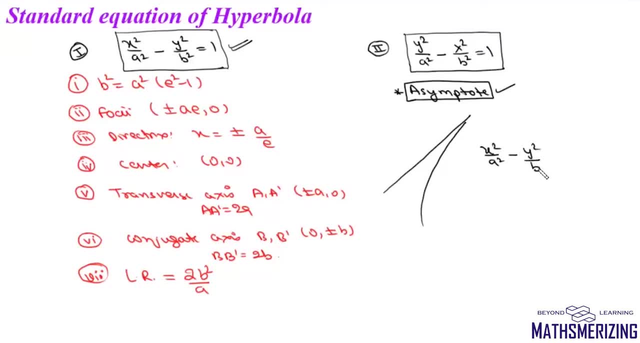 x square upon a square minus y square upon b square, and it is equal to 1.. And we need to find its point of intersection with this line, which is: y equals mx plus c. So what we will do is we will replace y with mx plus c, So we can write. 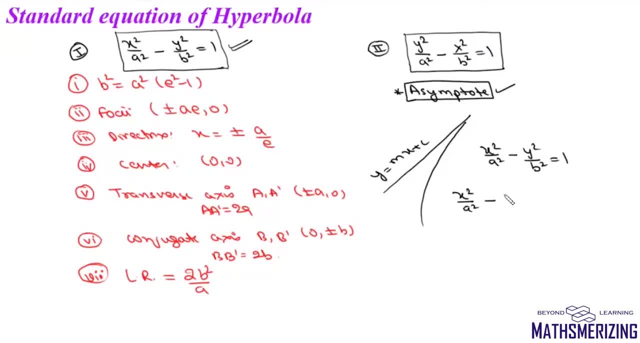 this equation: as x square upon a square minus mx plus c, whole square upon b square equals 1.. So we can write this equation as b square, x square minus a square, m square, x square plus twice mcx plus c square, and this is equal to a square b square. 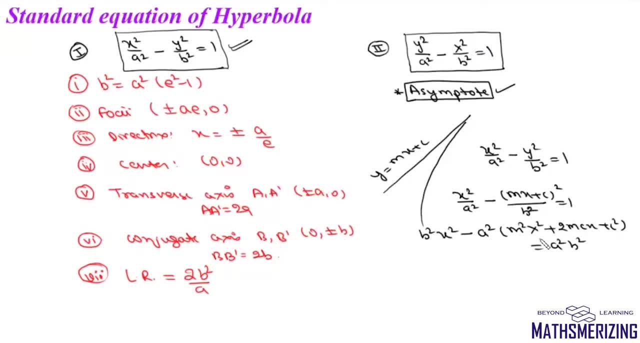 So we can write this equation as a quadratic equation in terms of x. So we will write this equation as b square minus a square, m square, x square minus 2, a square m into c, into x, and then minus a square, and it will be b square plus c square equals to zero. 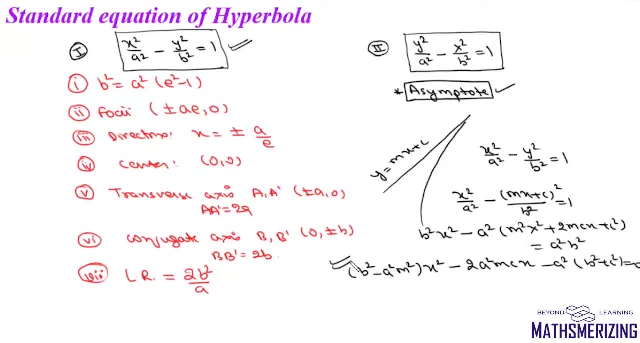 which is a quadratic equation in x. Now we know that this line is an asymptote and, by definition, asymptote is that line which intersects the curve at infinity. So it simply means this equation should have two infinite roots. Now we know that any equation which is of the form, 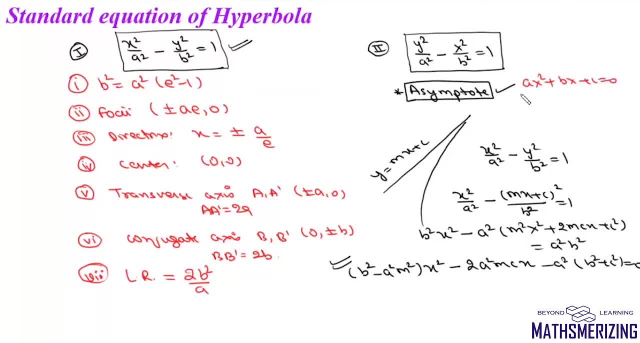 ax square plus bx plus c equals to zero- will have two infinite roots When a is zero and b is zero and c is unequal to zero. So we will put a as zero. we will get b square minus a square m square, it is zero. and then minus 2, a square m into c is also zero. 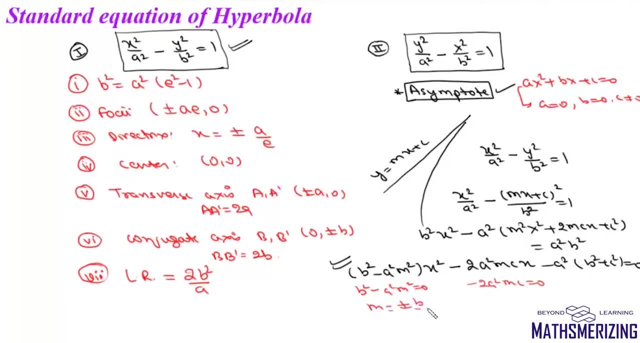 So from here we will get the value of m as plus or minus b upon a and we will get value of c as zero. So this line which intersects this hyperbola at infinity, will be given by the equation: y equals mx, m, in this case, is plus, minus b upon a, x and the value of c is zero. So equation of asymptotes. 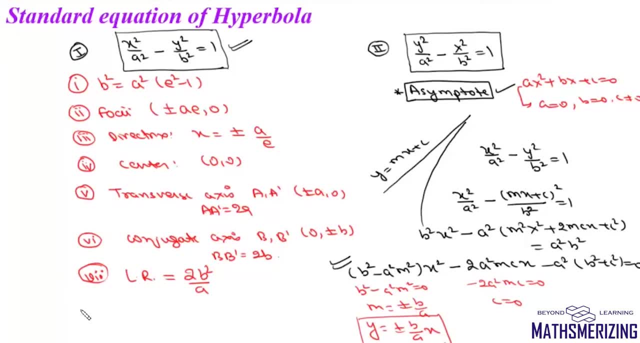 is given by y equals plus minus b upon ax. So this eighth one is equation of asymptotes. and equation of asymptotes is simply y equals plus minus b upon ax, and we can also write endpoints of latest rectum. So endpoints of latest rectum is given by: 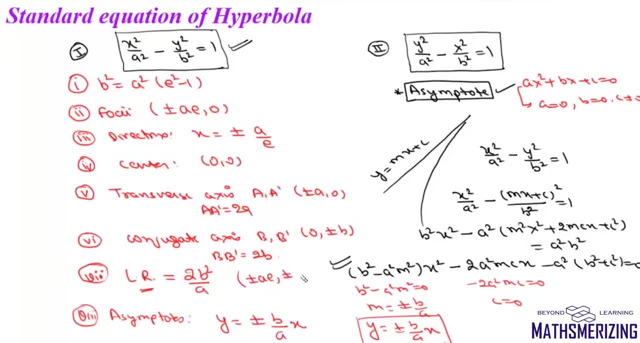 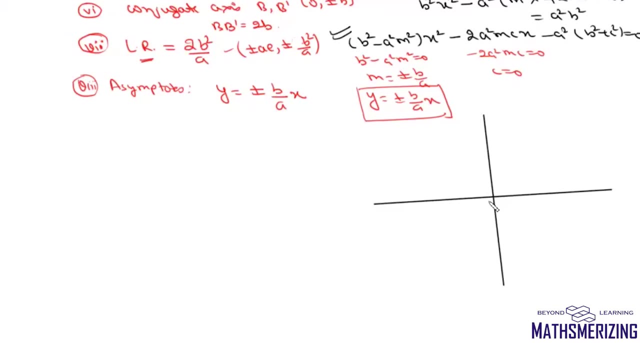 plus minus a and plus minus b, square upon a, which is same as that of ellipse. Now we will draw this hyperbola, So we will draw the axis Center at origin. Now, first we will draw these two asymptotes, So we will draw two lines. 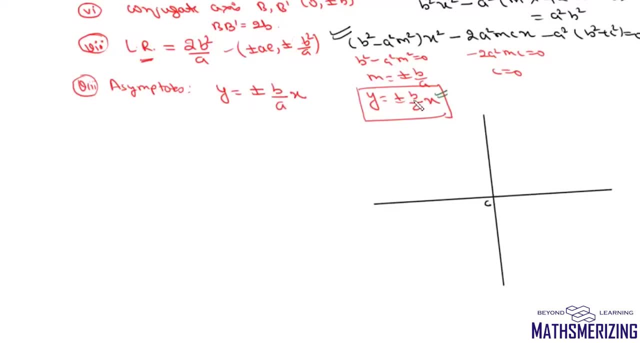 passing through origin and whose slope is b upon a and minus b upon a. So on this line there is a larger endpoint of a certain point, the unit length, which is just a little quite limited, which we are going to be adding all connection lines and multiple of them, and 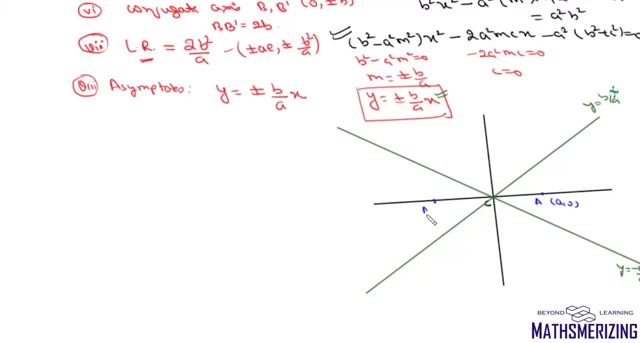 so on and so on. So we will draw two lines passing through from a andm, And then we enter all these Justin economists findings as close festing points here, as once you will add roots to it, And then we have b and b dash, which is 0 comma b and 0 comma minus b. 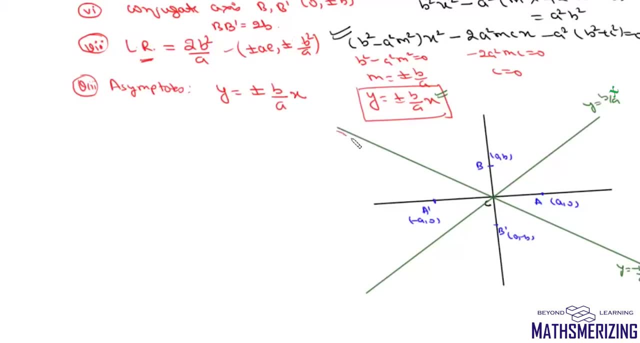 So now we can draw this hyperbola. Now, basically, hyperbola will have two branches, So we'll draw one branch on the left and we'll draw other branch on the right. So this is how we can draw a hyperbola. 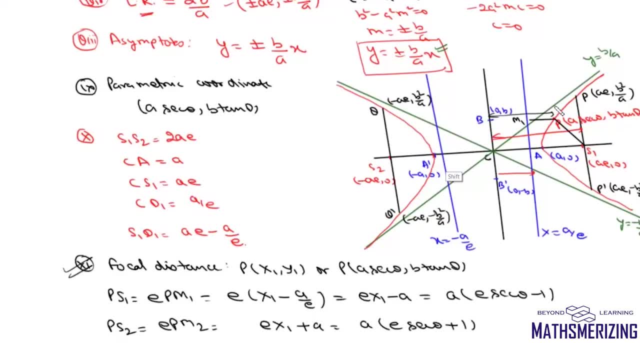 Now there is this one more thing about this asymptote, and that is: if there is any line which is parallel to asymptotes, then it will intersect the hyperbola only at one point. So if we ever take a line which is parallel to asymptote of this hyperbola, then that 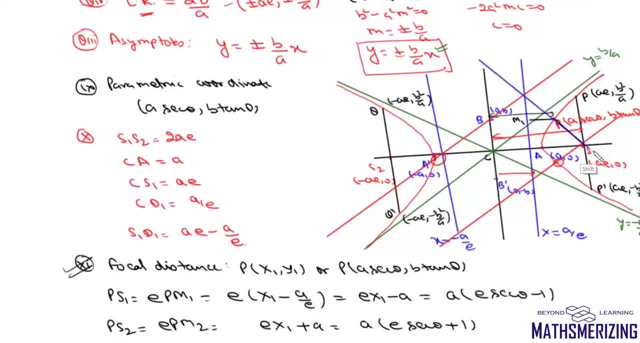 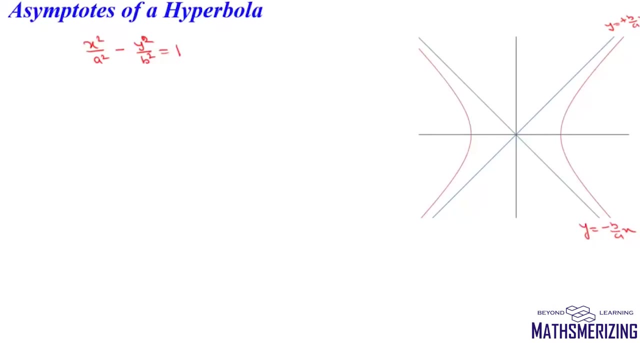 line. it will intersect this hyperbola only at one point. All of the lines, either they'll not intersect or they'll intersect hyperbola. So we can draw hyperbola at two distinct points. Now this first result is suppose we have any double ordinate of a hyperbola, which is p. 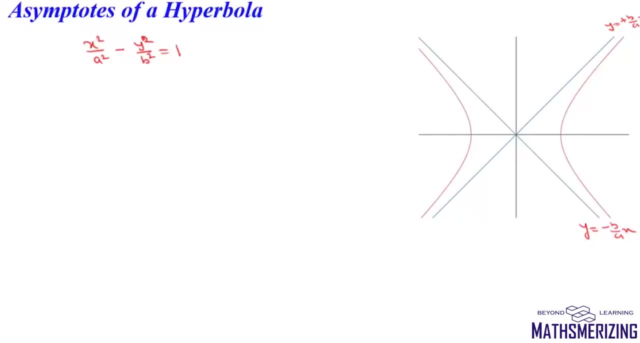 and p dash And if it is produced both ways to meet the asymptotes in q and q dash, we need to prove that pq into p dash, q is equal to b square, So we'll draw double ordinate. And this is p and p dash and it is extended to meet the asymptotes at q and q dash. 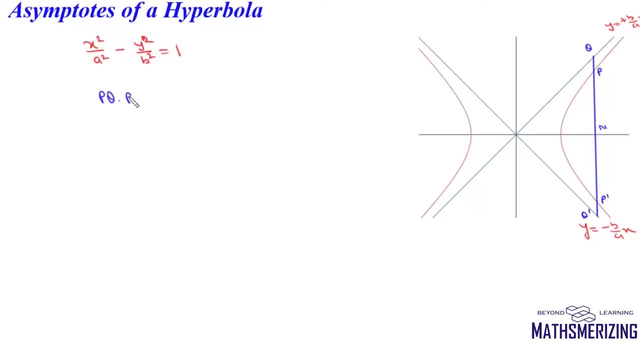 We need to prove that pq into p dash q. it is equal to b square. What we'll do is we'll take this point p as a secant theta and b tan theta, And now we can write p dash s. So we'll take this point p as a secant theta and b tan theta. 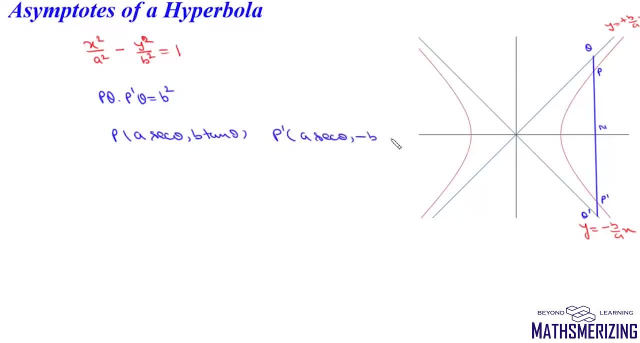 And now we can write p dash, s. So we'll take this point p as a secant theta and b tan theta. Now we'll find this corresponding point q. Now we know that this q it lies on this p, p dash, So it's x coordinate will be seen. 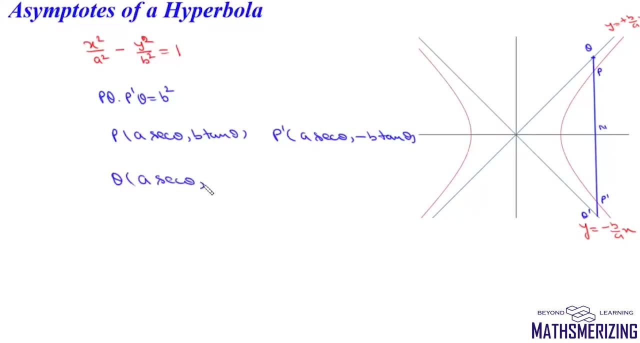 So it's x coordinate will simply be a secant theta And we'll put x as a secant theta. we'll get y as b secant theta. Now we'll find pq. Now pq is basically physical distance between Q and P. So it will simply be B secant theta minus 10 theta and we will 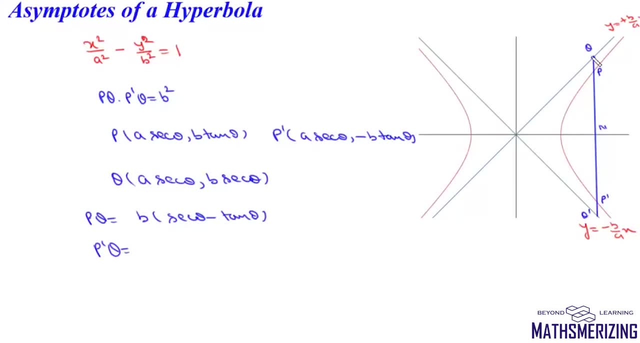 find P dash Q. Now P dash Q will be: it will be B sec theta and minus minus, plus B tan theta. So it will be B secant theta plus tan theta. So we will multiply them. we will write P Q into P dash Q. it will be B square and then it will be secant square theta, minus. 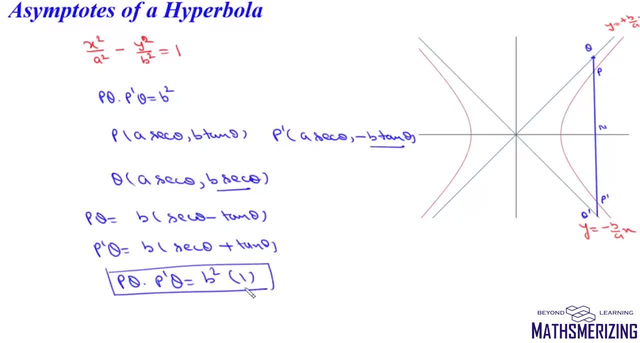 10 square theta, which is simply one. So we can write that this product of P Q into P dash Q will be B square, And in the same way we can also prove that this P Q dash and P dash Q dash will also be B square. Now the second result about asymptote of a hyperbola. 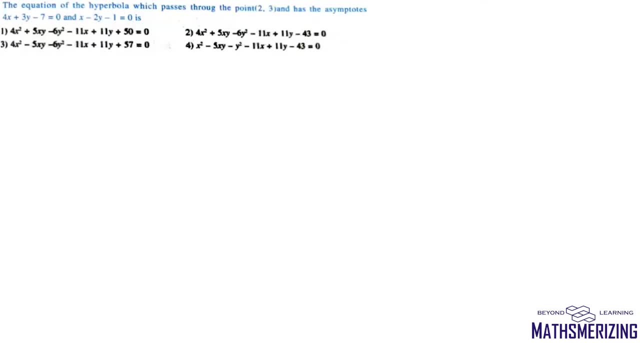 is equation of pair of asymptote and equation of hyperbola differs only by a constant. So if we have equation of hyperbola which is, say, S equals to 0, and if we have to write equation of P of asymptotes, then that equation simply will be s plus lambda equals to zero, and in the same way 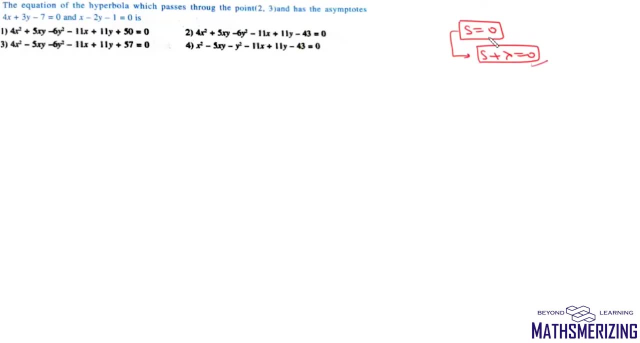 if we have two asymptotes, then we can multiply these two equations to get equation of pair of asymptotes, and then we can add any constant to get equation of hyperbola. now say, for example: suppose we are given this question, which is the equation of the hyperbola which passes through? 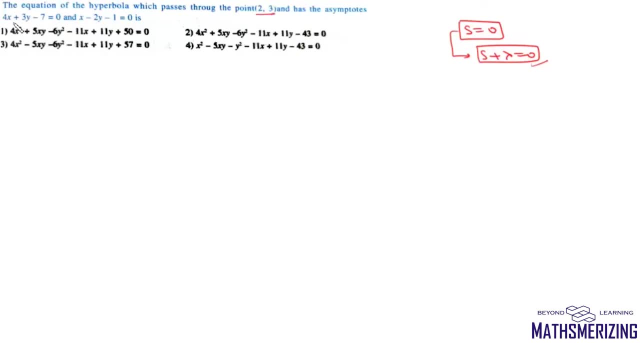 the point 2, comma 3, and has the asymptotes 4x plus 3y minus 7 equals 0, and x minus 2y minus 1 equals to 0. is so first what we'll do is we'll find equation of pair of asymptotes. 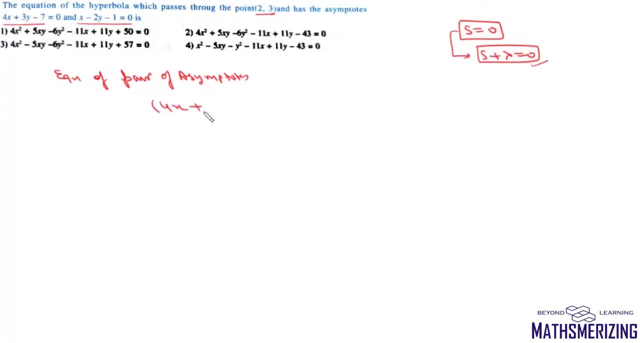 so equation of pair of asymptotes simply will be 4x plus 3y minus 7 into x minus 2y minus 1 equals to 0. now we know that equation of hyperbola and equation of pair of asymptotes only differ by a constant, so so we can simply write equation of hyperbola as: 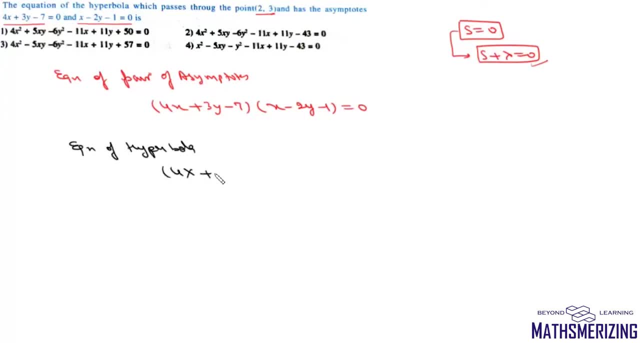 this equation of pair of asymptotes, which is 4x plus 3y minus 7, into x minus 2y minus 1, and then plus c equals to 0. so we have just added a constant to it. now it is given that this hyperbola, it passes through. 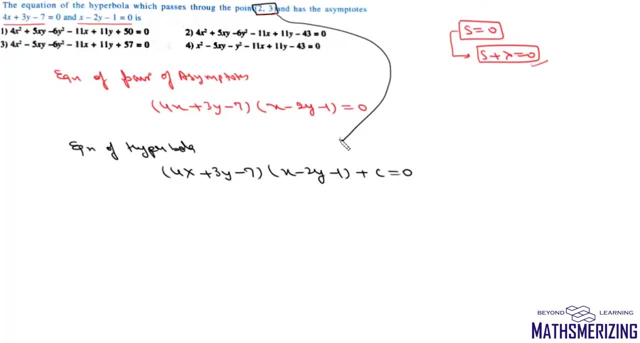 this point, which is 2 comma 3. so all we need to do is we just need to put the value of x and y in the equation and then we can get the value of this c, and we'll simplify, we'll get our answer, so we'll.